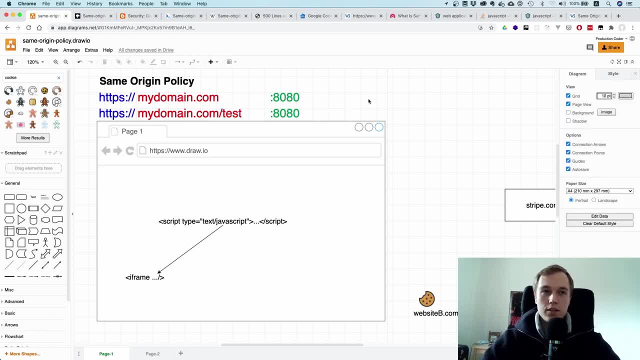 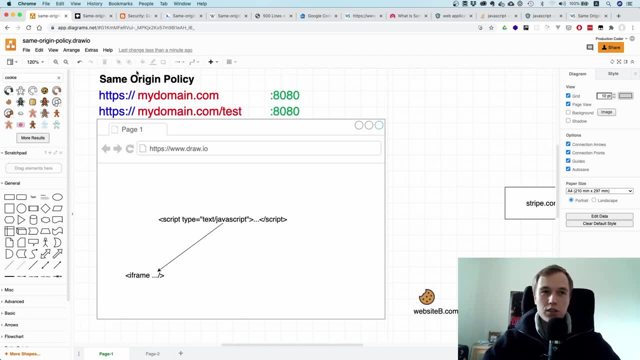 they are considered to have the same origin, and this is basically the main concept that we're talking about when we're talking about this policy. yeah, so let's maybe talk about what kind of problem this thing is trying to solve, and then we will talk about how it attempts to do so. so, if we look 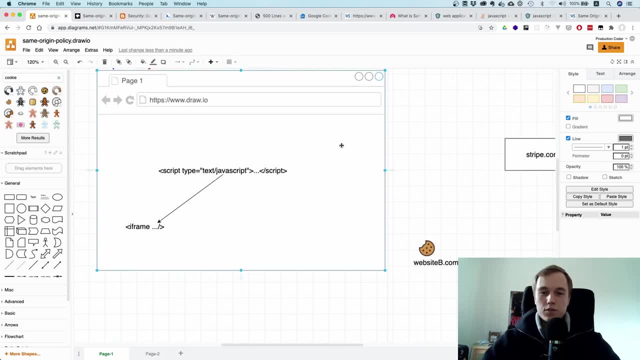 at the modern browser, then you can do a few things. so, for one, you can have multiple tabs, just like i have over here. you can have multiple tabs with different origins. right, you might be on draw- oh, maybe you're on twitter at the moment, or you have like some documentation open, and what you definitely don't want is you. 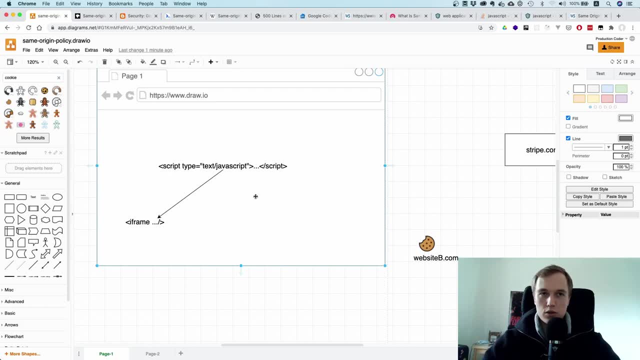 don't want some javascript that runs on one website. so, for example, here on draw io to access like the dom or another website that you might have opened in another tab. so say you're currently locked inside of your online banking account, then you don't want like. 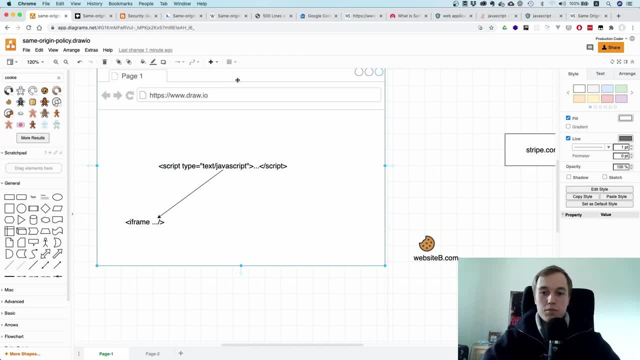 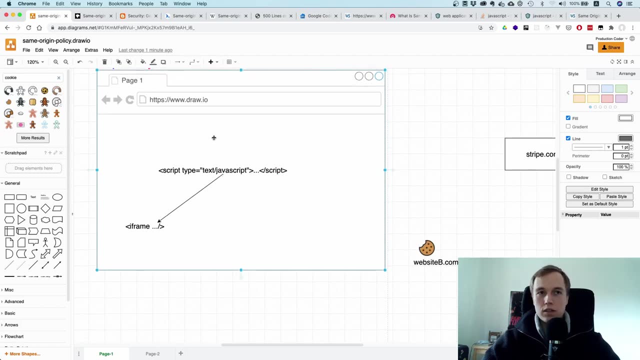 any website to be able to access like your banking website, right, and this is basically the first use case. so you have like different tabs or different tabs where the origin is different, and then you don't want like this cross origin access. now, just as a side note. 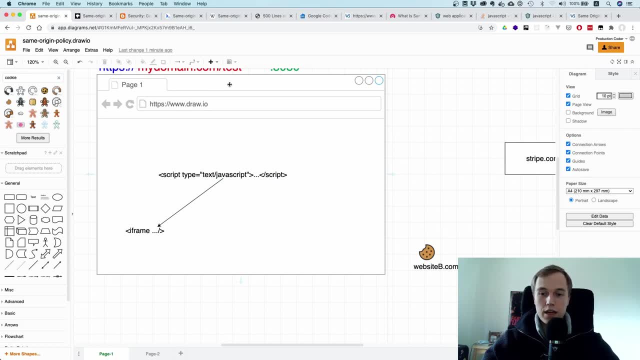 you can actually access document that is in a different tab, as long as it's the same origin and you have a reference to it. so if you programmatically open a tab and it's the same origin, then you can actually access and manipulate the dom. just saying, because otherwise it. 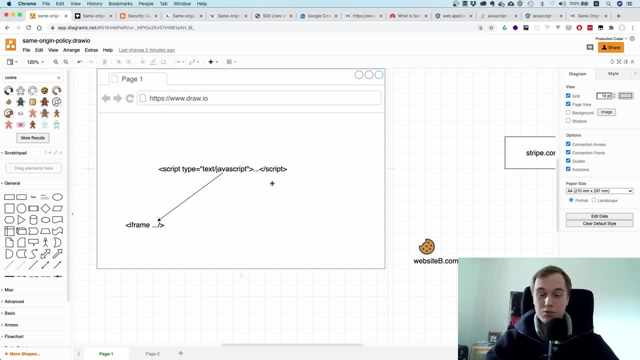 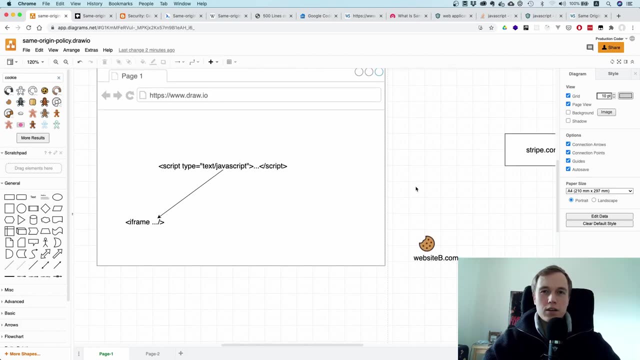 might sound as if this is totally impossible. no, it's not, but it's very restricted, okay. so this is like a first case, and what you, or what's also important on the web, is that there are a few items or artifacts that you have that you don't want to share. so say you have like a session. 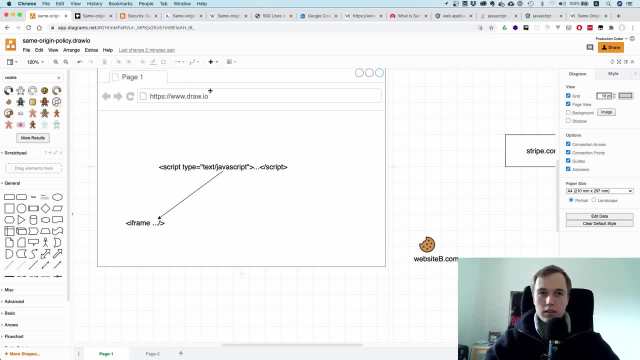 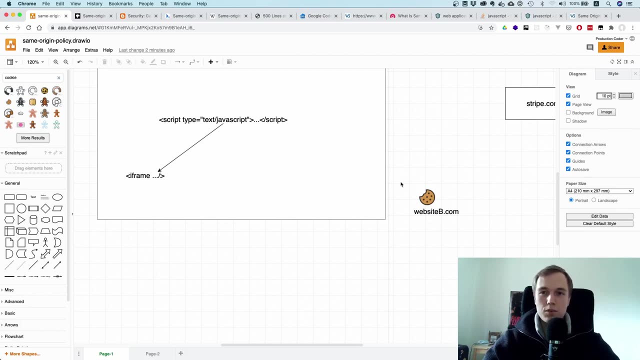 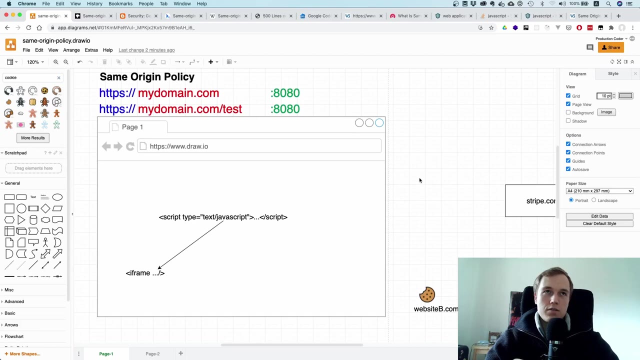 cookie from websitebcom, then you don't want, like the draw io website, to access this cookie, right, because this cookie might be critical. it might contain some important session information. okay, so in principle, the same origin policy says: hey, if we have like different origins, then we need to be very careful with what scripts are allowed to do. and that is the next important. 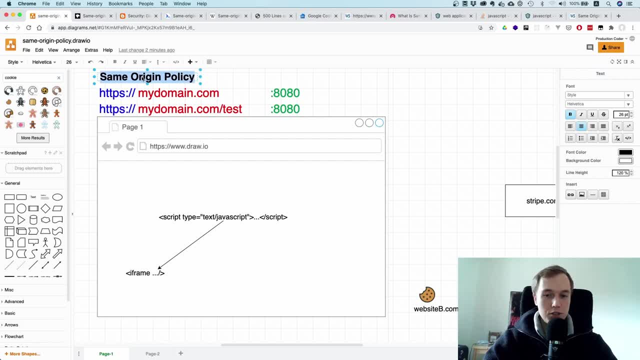 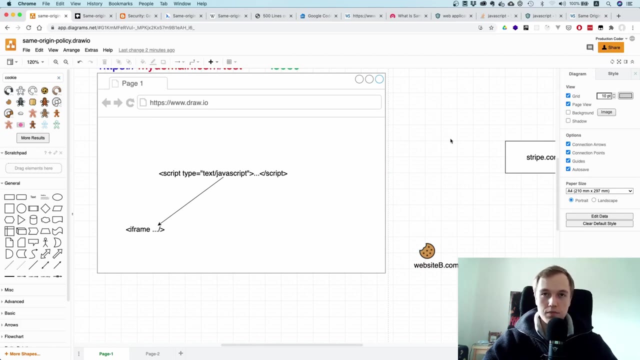 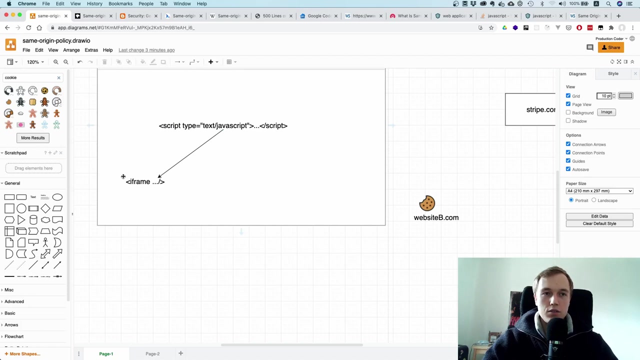 part the same origin policy. it's not about images, it's not about css or about like anything else, it's just about scripts. so in other words, it governs what a script on one origin is allowed to do. so let's make an example. okay, let's say you have a website say draw io, and you have an iframe here. 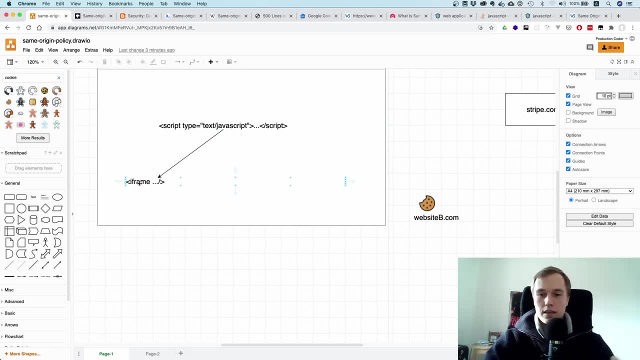 i don't know, maybe you. this is some marketing widget right where you can enter your email address and then you can sign up for a newsletter, and this is by some other company or by some email marketing company. so the origin of this iframe, which is like a document or its own website in 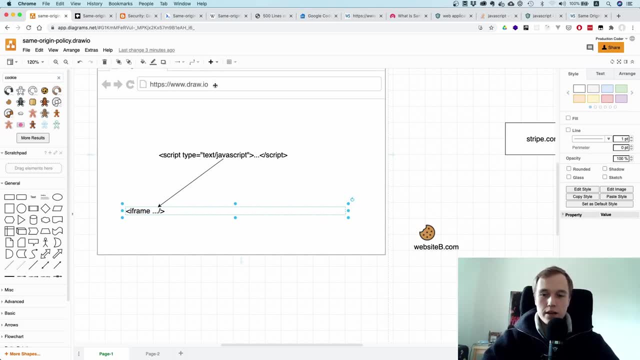 itself is different than the one from draw io, and what this means is, as we have learned before, if it's like different origins, then it, like the browser, needs to be very careful with what it allows a script to do. so if you have a script over here, then obviously the origin of that script is the current url, which is draw io. 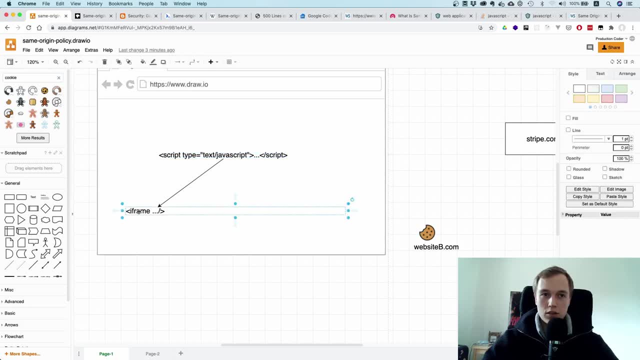 and now, if you access, if you try to access the content of this website here, which happens to be in the same document because it is embedded, then, like you, can't really do much, so it's not do whatever you want with this iframe, so it's it's not as restrictive in the way that it says you're. 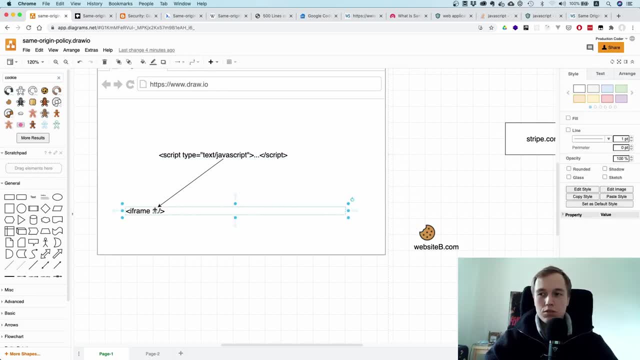 not allowed to access it at all. you can't do. you cannot do much, right, and this is obviously on purpose, because just imagine, like this is some phishing website and this iframe is like your banking website. okay, and this is just a custom script. so in that case, if this script could, 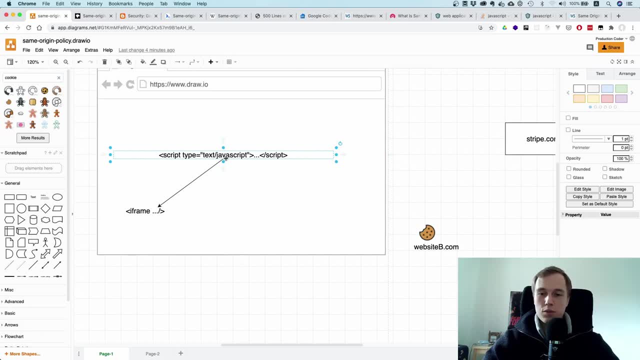 access the website. then you would enter your username, your password. the script could just read it out and consult you from your id and then it's stitch, just clickруж enough quickly. so you, yeah, your credentials- are on. some are gone, like some hackers stole your credentials, cool. so in that case, it's clear that the origin of this script is. 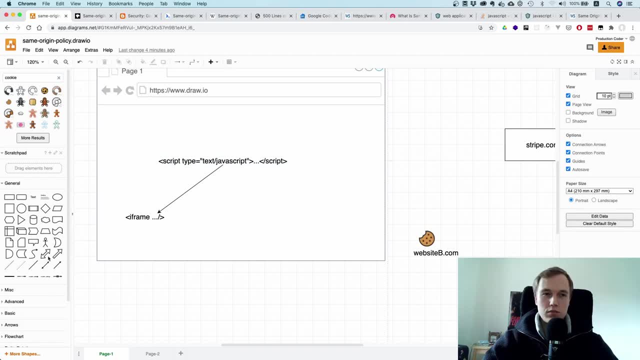 like drawio. and what I also wanted to point out, which might be like a little bit surprising maybe at first, is: let's imagine I pull this script in from another, from some CDN so say: it's like stripecom or so alright, so I take this thing and I pull it from in from stripecom. then you might say, oh well, but 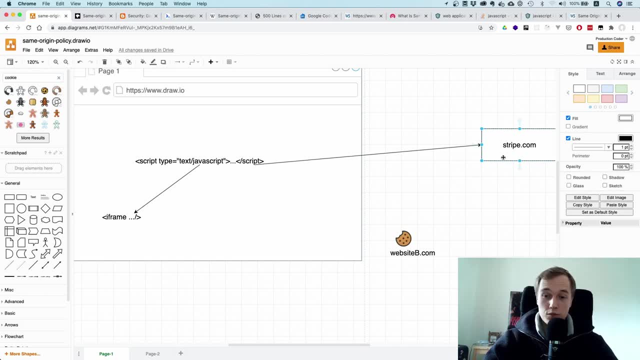 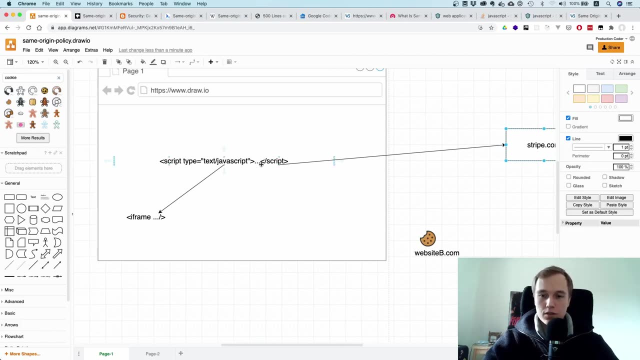 hold on a second. like this script. it's originally from stripecom, so its origin is stripecom, and that is actually not correct. so the origin of a script, or what determines the origin of the script, is the document in which it lives in. so even though this script might be pulled from a different website, 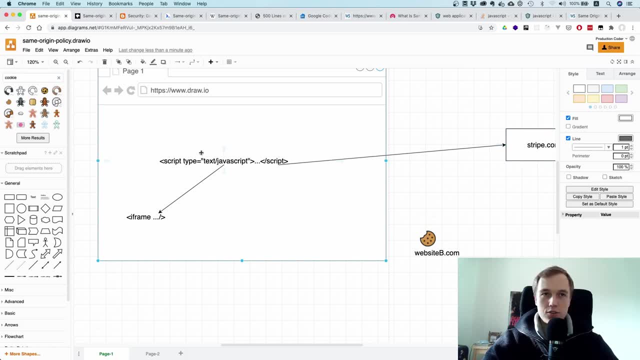 from a CDN. its actual origin is the document in which it is located, which is at the moment drawio. so that means the script that you pull in can do pretty much everything with your DOM, except, like as we said before, accessing this iframe, because that would be cross origin operation again. right, and that. 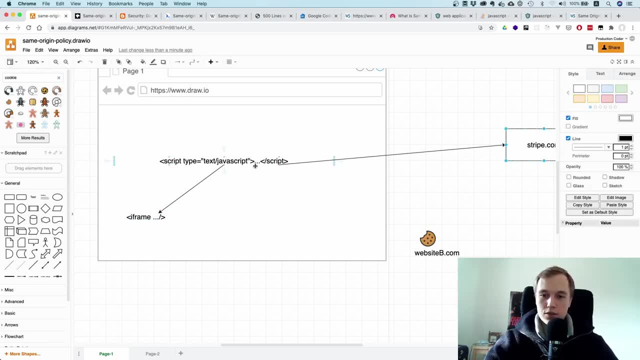 also makes sense. just imagine if we were to consider this as a different origin. like this script here. how would we have, like all these services that you have on the web? right, you have some service provider, you pull in the script and it does whatever you want to do. and then you pull in the script and it does. 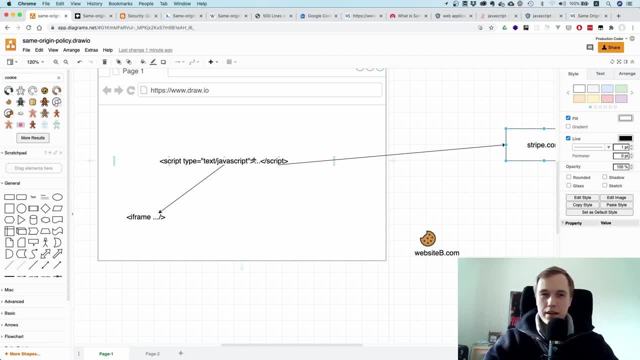 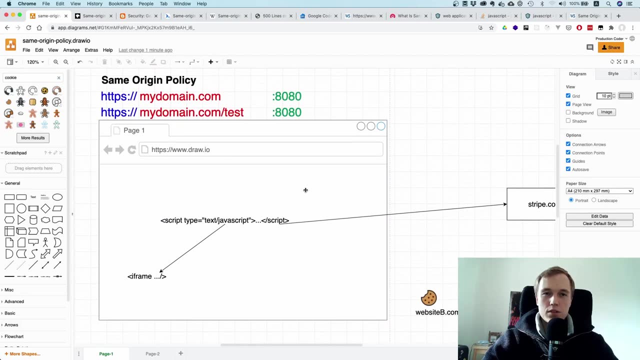 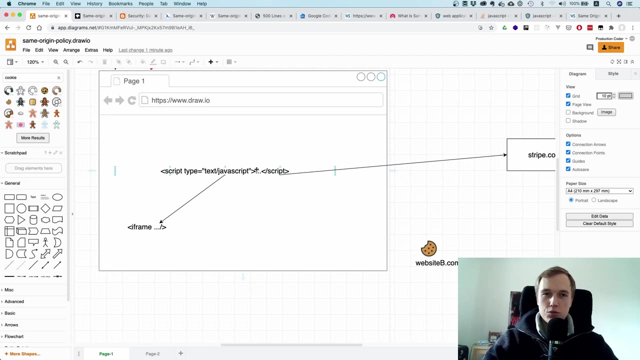 whatever you want it to do. so it makes sense that this is the same origin. okay, yeah, so that is, in principle, what the same origin policy is. there are a few other things, so, for one, the same origin policy says that you are allowed to- in principle allowed- to write out requests. so that means if you load a script or if 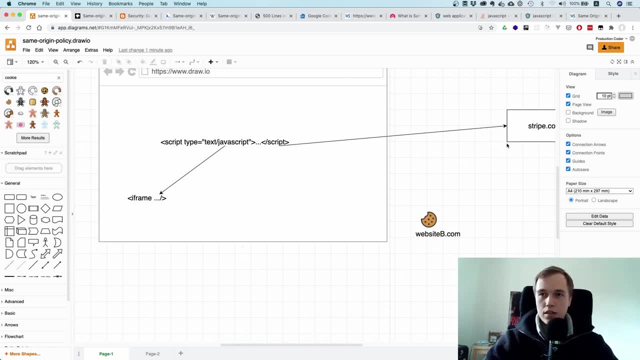 you have a script and it tries to access a different origin. it tries you to access a different origin. it tries you to access a different origin. it tries you to try to submit a form or you, I don't know. you make a post request, for example. this is in principle possible. a few HTTP verbs are not possible, so put and. 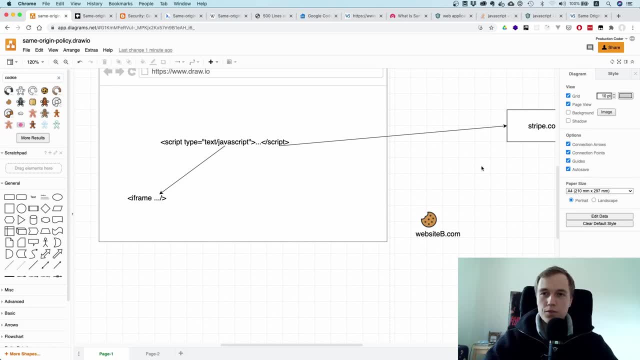 maybe patch, I'm not sure, but put, I'm pretty sure. so if you have one script that attempts to make a put request to another origin, and then this is problematic and right now we're only talking about the same origin policy, right? so this is important because in the real world this would 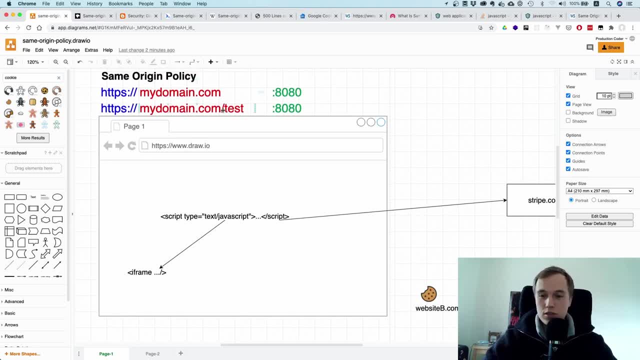 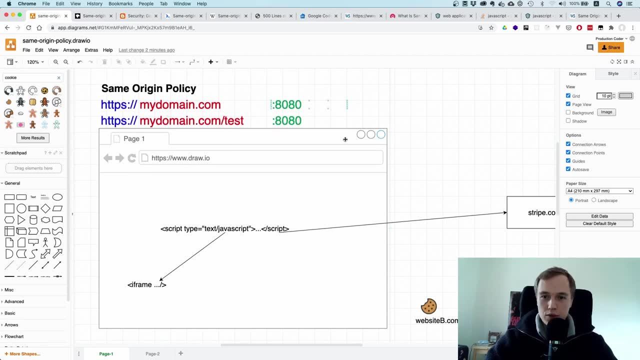 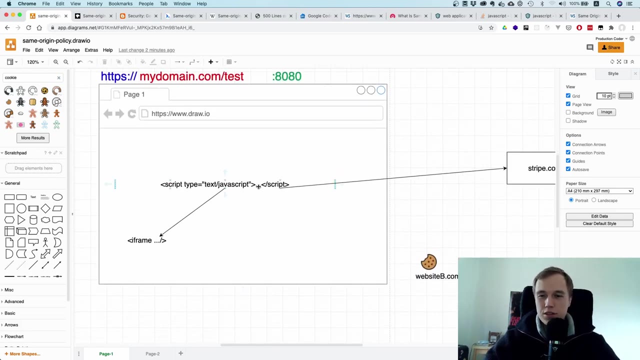 obviously not work because, apart from the same origin policy, you also have something like course, and that would most probably prevent you from doing something like that. so, at the moment, what we are explaining here is really the purest same origin policy. yeah, so, as we have seen, like this same origin policy, sometimes it's too.